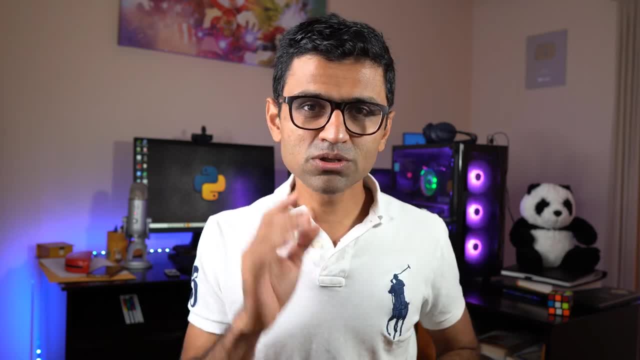 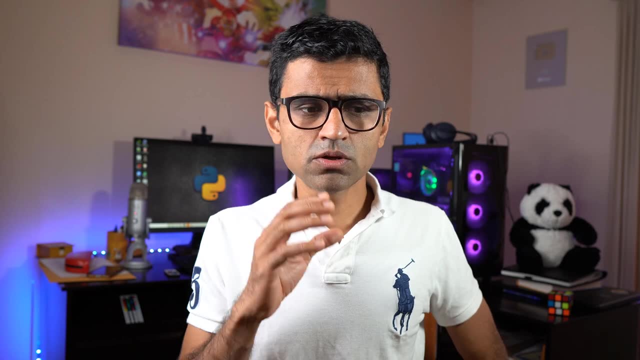 If you want to build a career in natural language processing domain, you need to have a knowledge of BERT, which is a very popular language model by Google. In this video, I'm going to explain you in a very simple language, as, if you're a high school student, you can also understand it easily. 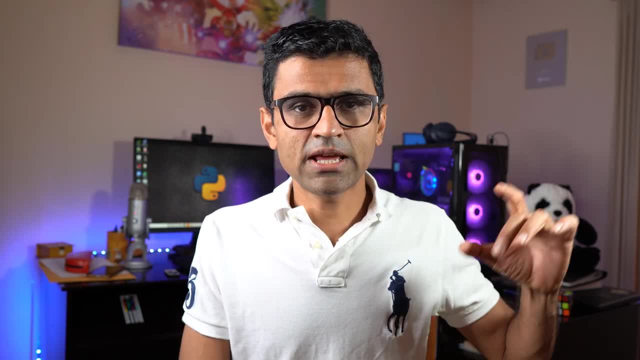 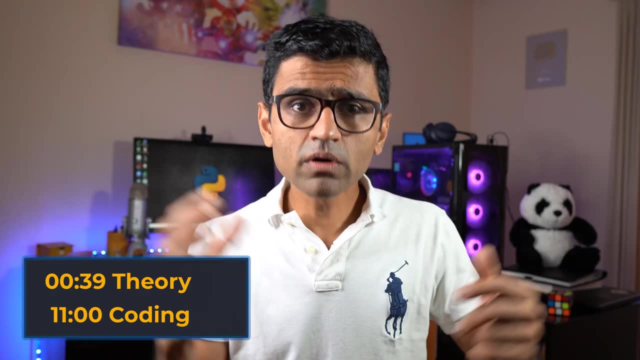 What is the point behind BERT, How BERT is used in NLP tasks. We will not go into details of transformer architecture etc. But we'll have an overview of how BERT works. basically the BERT model, the usage. 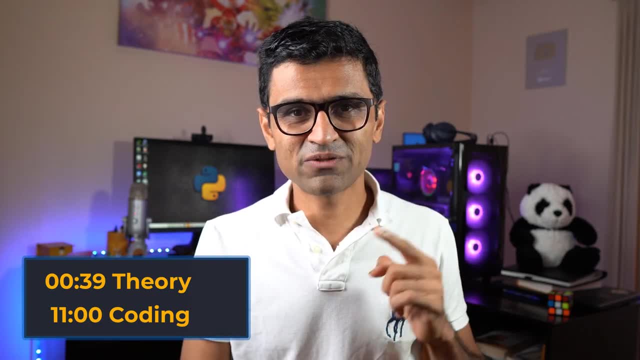 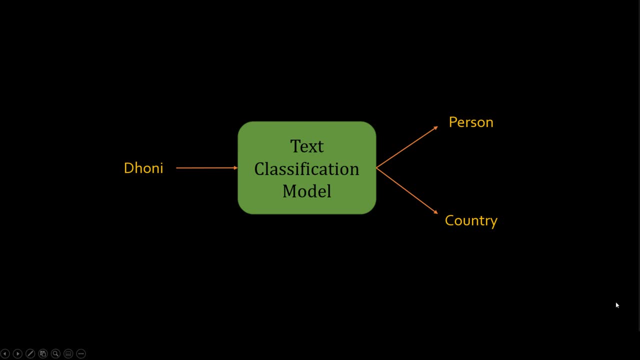 And we'll also write some code in TensorFlow and we'll generate some sentence and word embeddings using BERT. So let's get started. Let's assume you are working on a text classification task where the input to the model is a word and you want to classify that as either a person or 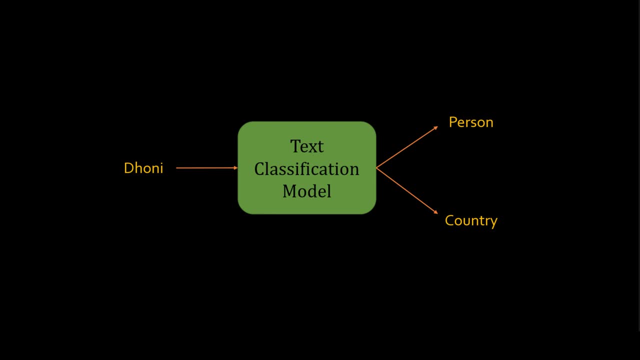 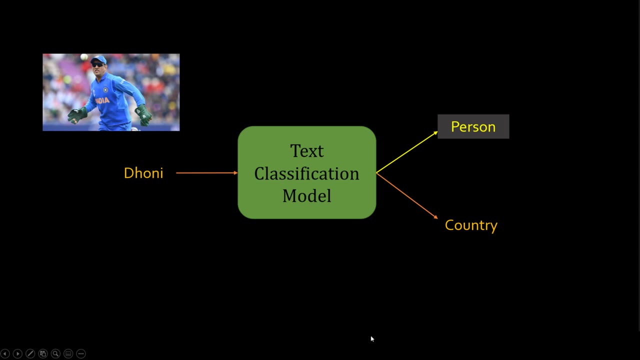 a country. The input word here is Dhoni, who is an Indian cricket team captain, and he's a person. So that's why you would classify the word Dhoni as a person. Now, the input is not an image. I'm showing you image just as a reference, but the input is only a word. 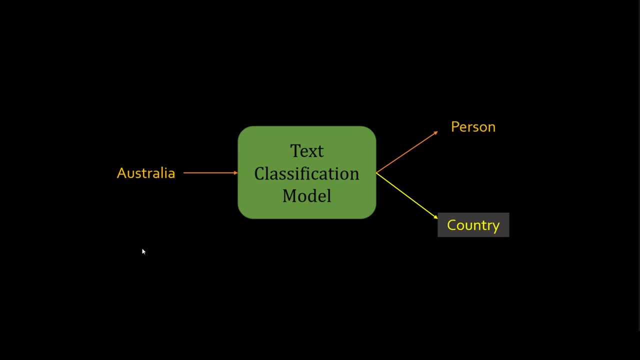 If the input is Australia, you would of course, classify it as a country. Mamudula, another Bangladesh cricket player, you would classify as a person. Now think about how this model would process the input word if it has seen Mamudula or Dhoni words before. 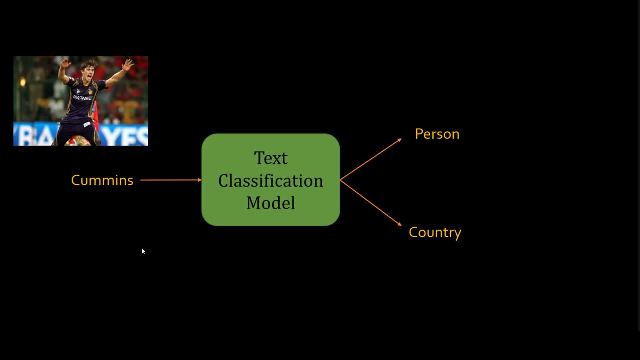 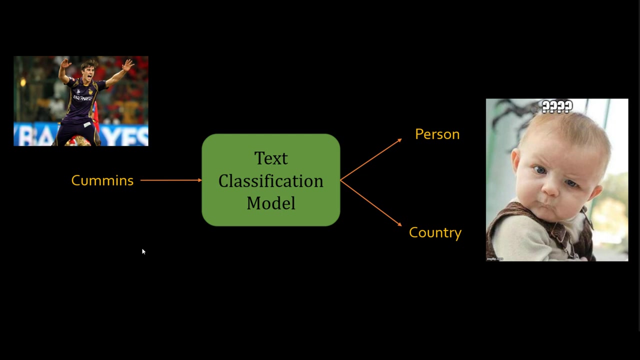 It can classify them as a person. But let's say the input word is Cummins. Now the word Cummins. how does the model interpret this word and can classify as a person? It is a little bit challenging, You know. you might be a little confused on how the model would do it. 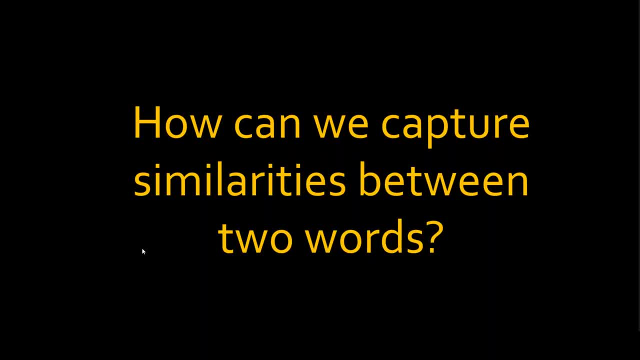 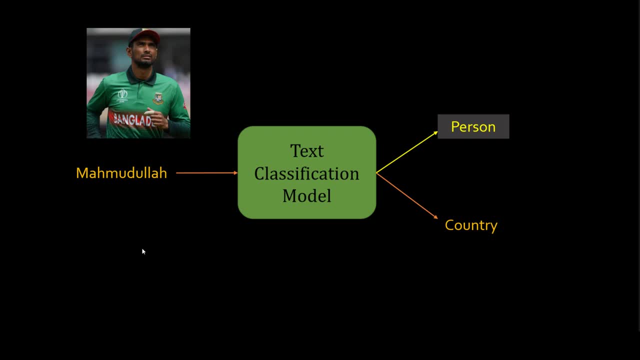 So the essence here is: how can we capture similarity? How can we capture similarity Between two words, similarity, as in Cummins is a person and a cricket player. at the same time, Mamudula is also a person and a cricket player. How can you say Mamudula and Cummins are similar, and let's say Australia, which is a country, and Cummins are not very similar? 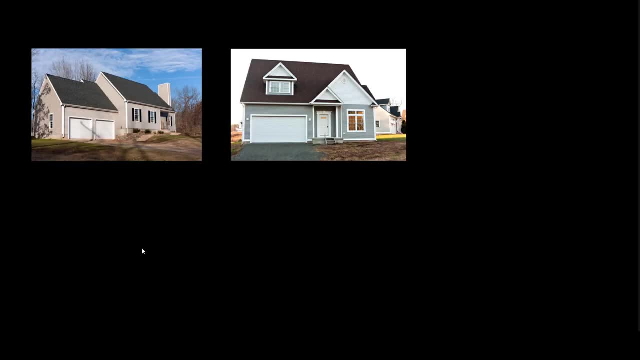 All right, let's think about if you have two homes. how do you say they are similar? You look at the features of the home. The features are bedroom area, bathroom, These two homes. you can say, yeah, they're kind of similar. 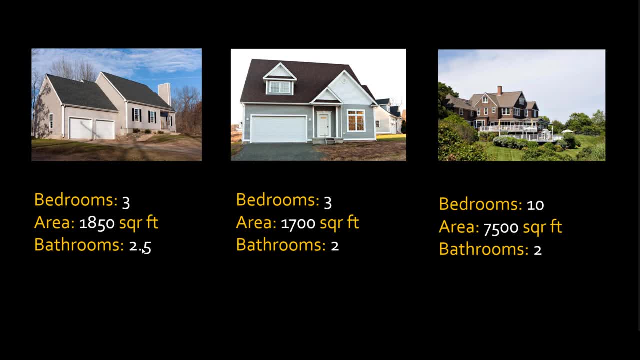 But when you have a third home, which is a bigger one, you know, 10 bedrooms, 7500 square foot, a pretty rich person would own this kind of home. You can say the second home and third home are not similar. 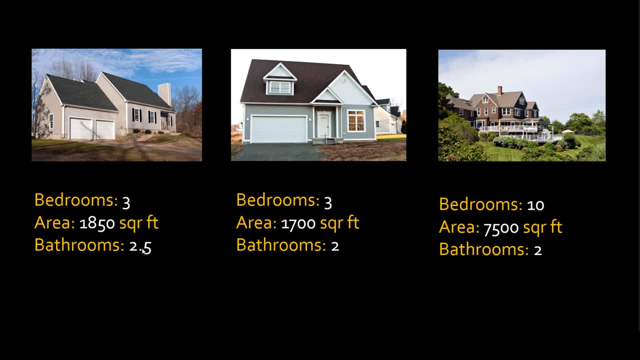 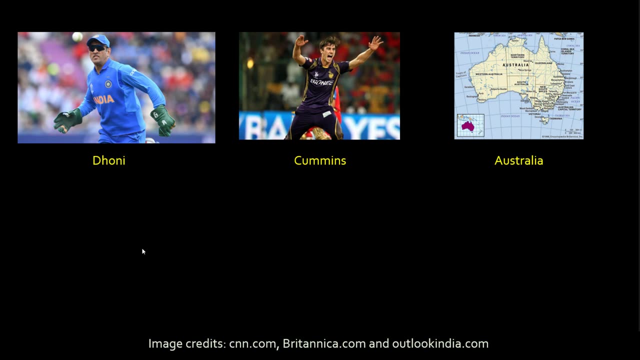 So if for an object which is home here, if you can derive the features, then by comparing those features you can say if those two objects are similar or not. Similarly, think about How you can translate these words: Dhoni, Australia, etc. 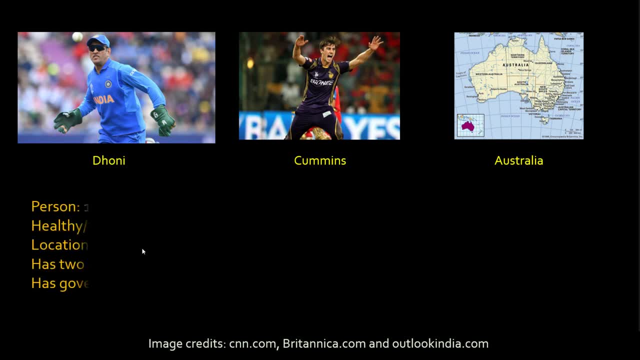 Into features. The feature could be this: Dhoni is a person, healthy and fit. The values are between 0 to 1.. 1 means like 0.9, means like really healthy. If it is 0.1, you know, say, a person who cannot run even one mile. 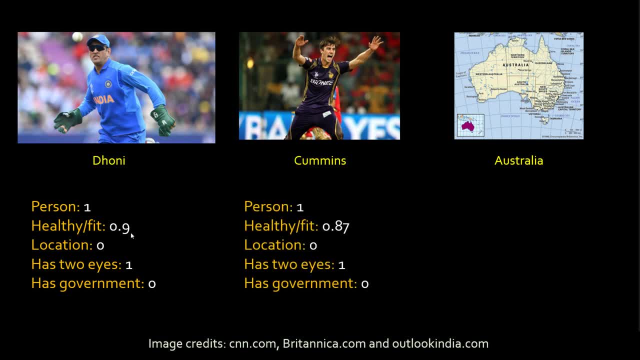 And if you compare these individual features you can say Dhoni and Cummins are kind of similar, but Australia is not Because they are similar, Because, see Australia- location value is 1.. Here location value is 0.. Person value is 0.. 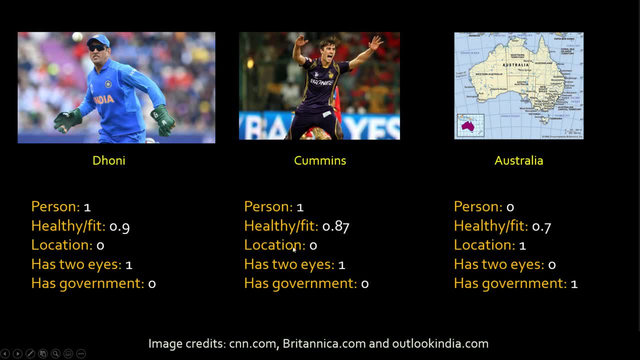 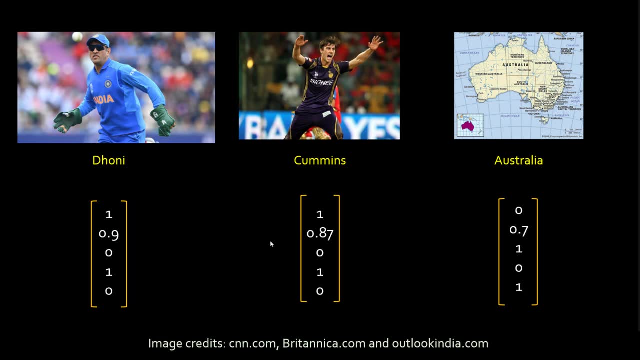 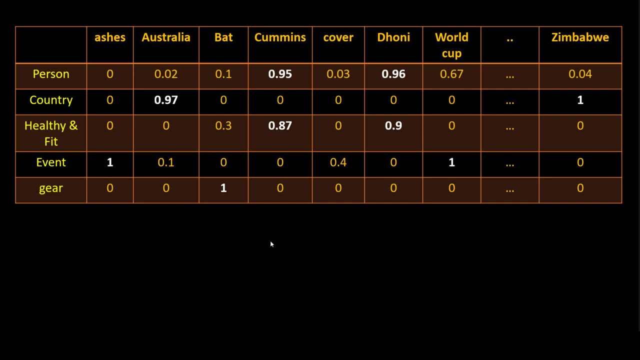 Person value is 1.. So if you take all these numbers and create vectors out of it and compare those two vectors, you can say that Dhoni is more similar to Cummins And Cummins and Australia are not similar. If you have doing, if you're building a model on, let's say, some cricket vocabulary, 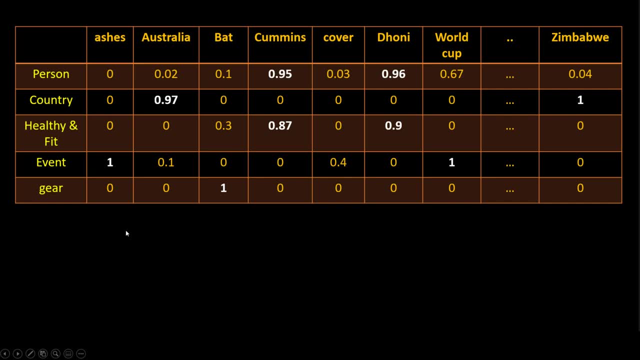 You might have words Such as essays, bad comments etc. And you can generate feature vector for each of these words. These vectors are called word embeddings And we have covered that in previous videos, So I recommend you watch those videos. But the essence here is that when you compare the feature vector or word embedding of Cummins and Dhoni, you will find that these two are kind of similar. 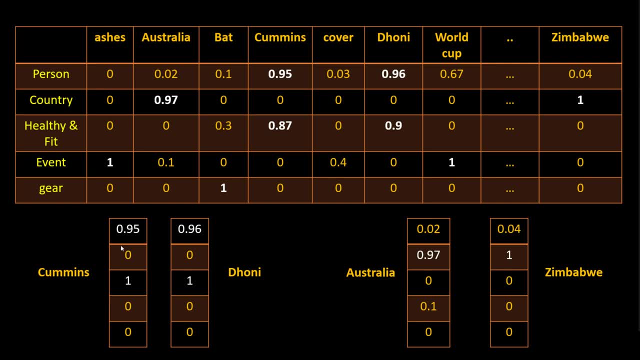 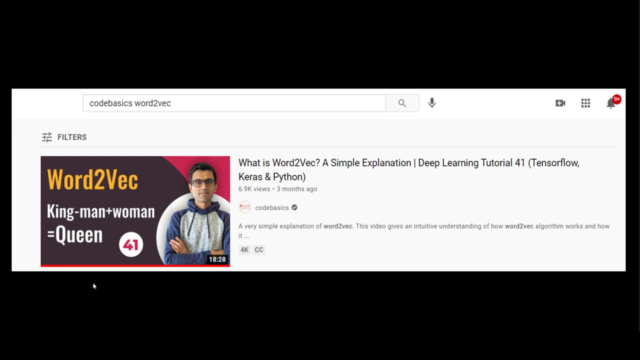 Whereas Australia and Zimbabwe are kind of similar. So those two are countries, those two are people. So this is a very powerful concept, And one of the ways you can generate the word embedding from the word is by using word2vec. So go to YouTube, search for codebasics, word2vec or codebasics, word embedding. 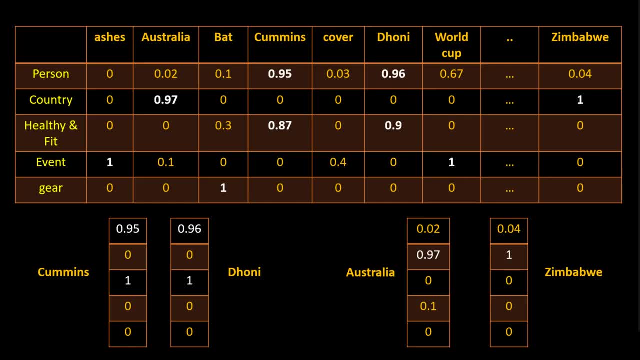 Watch those videos, You'll get a good understanding. Here we took these features individually, But in the real life the models can figure out better. The models can figure out these features on its own. It almost sounds like magical how they can do it. 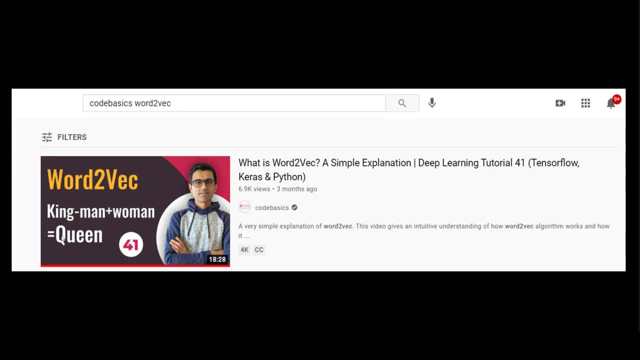 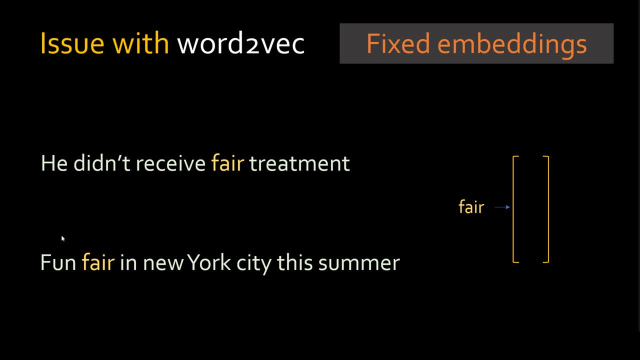 But it is possible. So for that you have to watch those videos. But the issue with word2vec is this: Carefully read these two sentences. The meaning of fair is very different in these two sentences. In the first one fair means, you know, unbiased, like equal treatment. 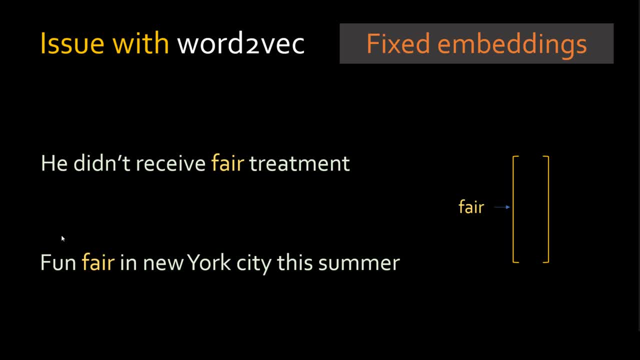 In the second one, fair means really carnival Or you know like fun activity. But word2vec will all generate a fixed embedding vector. Now if you use a fixed embedding vector in both the contexts then it's not right. 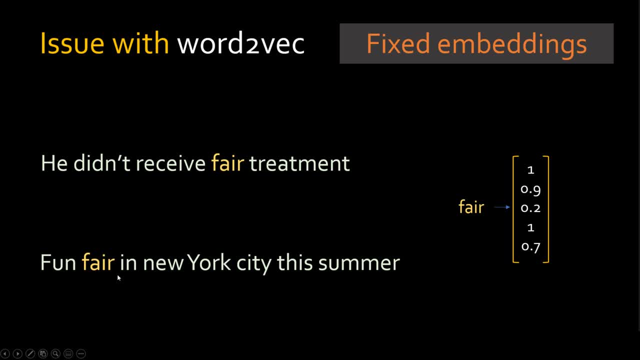 Because really the meaning of fair in both the sentences is different. So you need a model which can generate contextualized meaning of a word Meaning. you can look at the whole sentence And based on that you generate the number representation for a word. 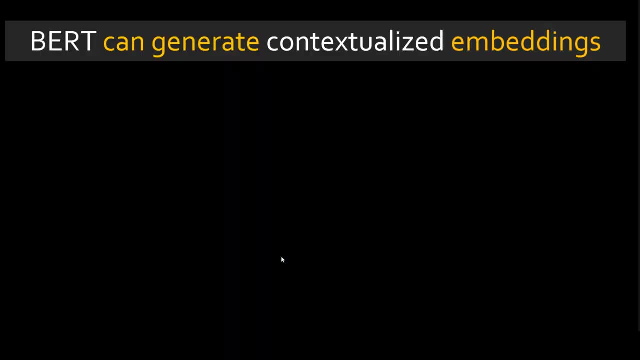 And word2vec allows you to do the exactly same thing. It will generate contextualized embedding Meaning. when you do these two sentences, you look at these word embeddings. Word2vec will generate it differently. Here is 1, here is 0.. 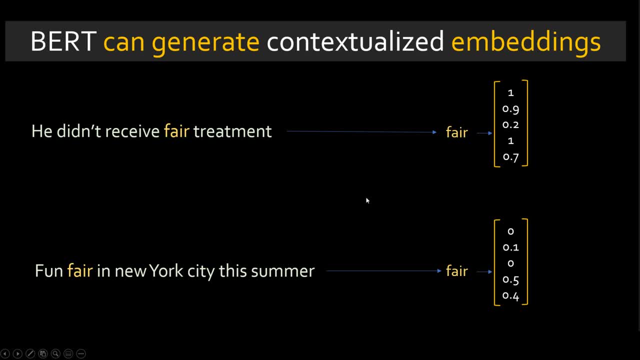 You can compare these two and they are different, But at the same time it will capture the meaning of a word in a right way, So that when you have a statement like Tom deserves unbiased judgment- Unbiased and fair are kind of similar. 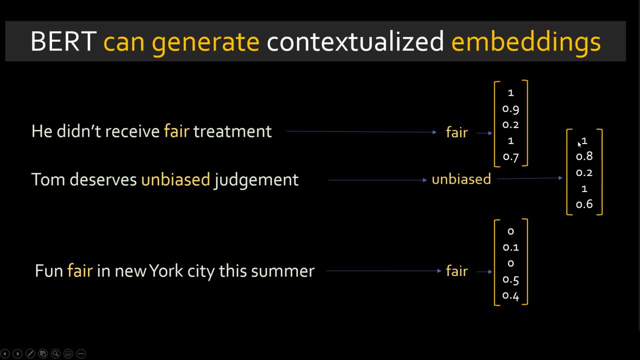 And you will see, it will generate a vector which is similar, See 1, 1,, 0.9,, 0.8, and so on. Similarly, when you have a statement like this, Carnival was packed with fun activities. 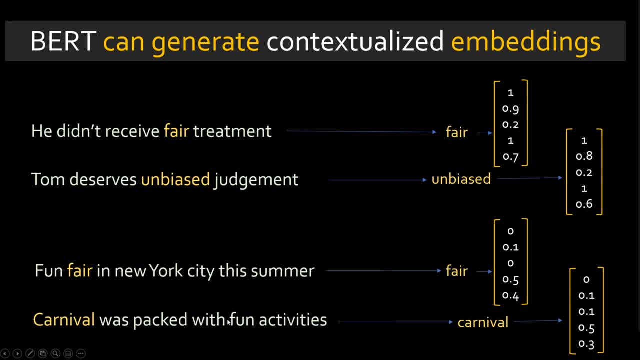 Carnival and fair are similar in these two sentences And it will generate similar embedding. So you can see, BERT is very, very powerful. It can look at the context of the statement and generate the meaningful number representation for a given word. 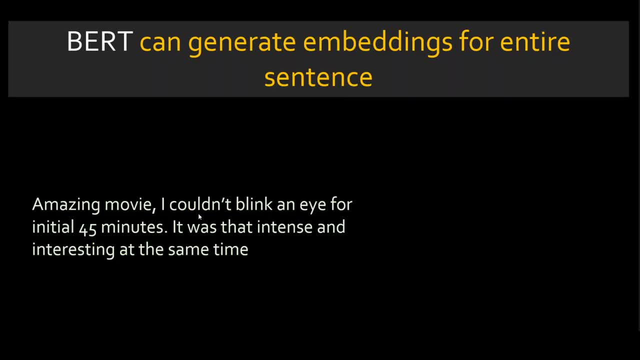 It can also generate an embedding for an entire sentence. Let's say you are working on a movie review classification task. For the whole sentence it can generate a single vector. Usually BERT will generate a vector of size 768.. It's just a number. 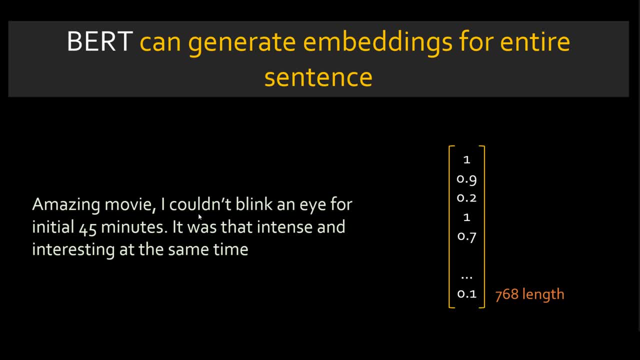 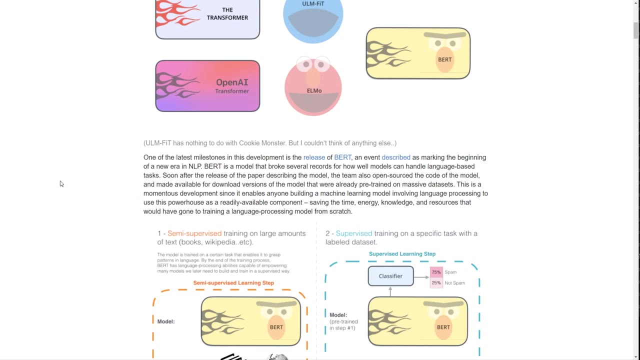 You know it can be anything, But usually they will generate this much, the vector of this much dimension. I came across this very good blog on BERT by Jay Alamar. He explains things in a visual way So you will understand more details about BERT. 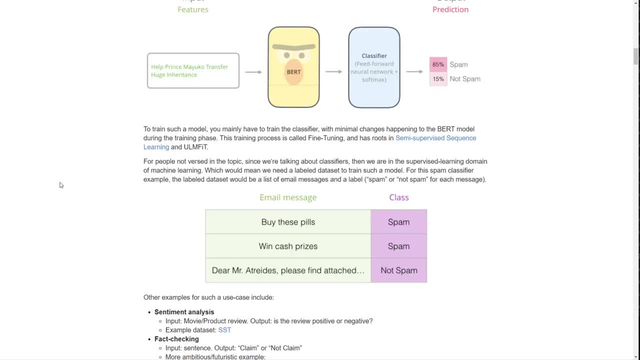 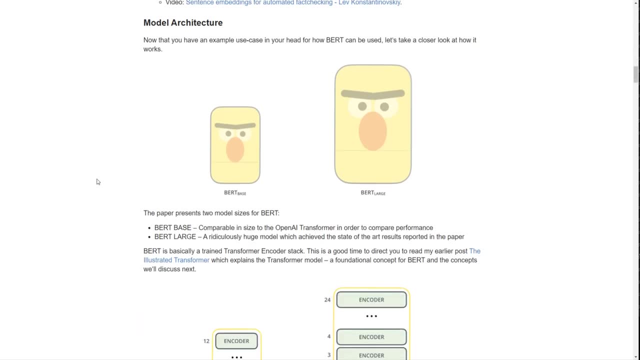 BERT is based on a transformer architecture which is the most latest one, as of 2021.. It is widely used in the industry. You have to know it if you are in NLP domain. There are two versions of BERT: BERT base and BERT large. 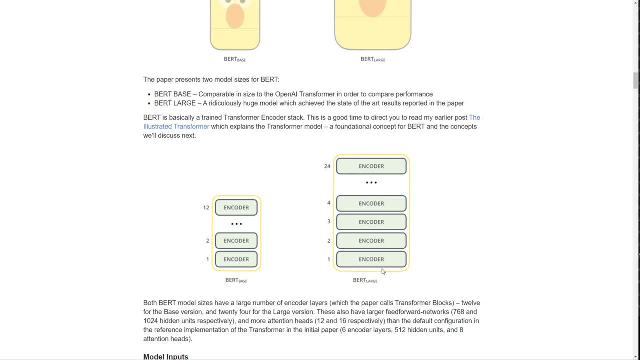 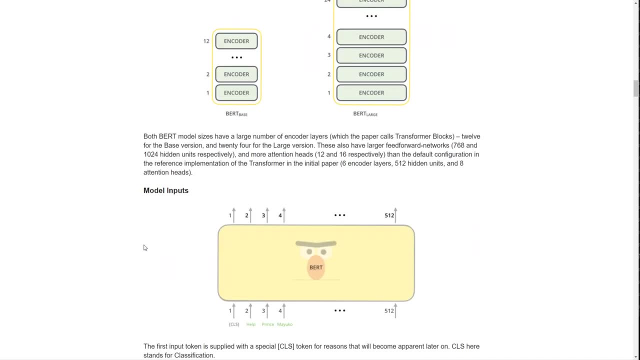 BERT base uses 12 encoder layers. BERT large uses 24 encoder layers. If you want to understand what these encoder layers are and details of the model itself, you can go through this article. But if you don't want to bother about it, 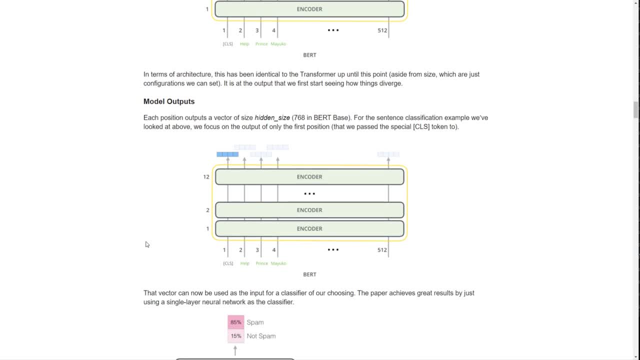 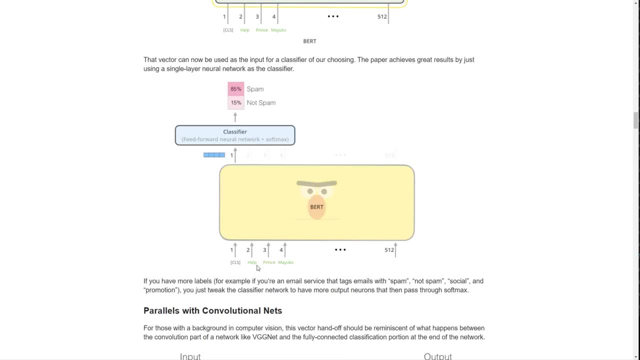 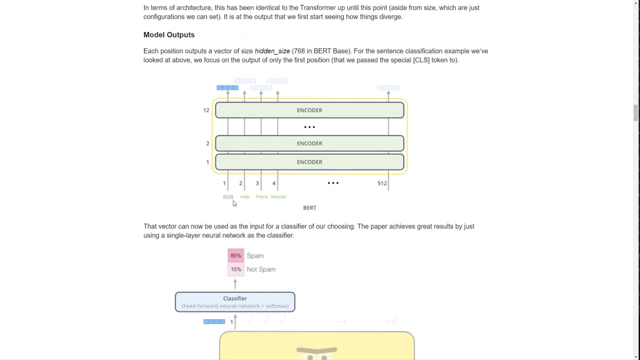 it is okay, You can just follow my presentation and kind of understand the purpose of the. you know the overview of BERT, But here in this article, see the BERT will generate First of all for BERT, you will have to use this spatial for a sentence. 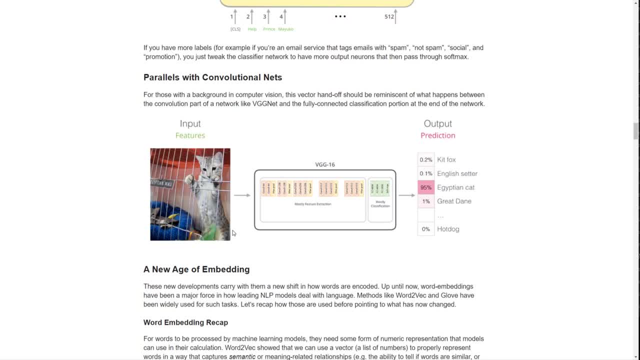 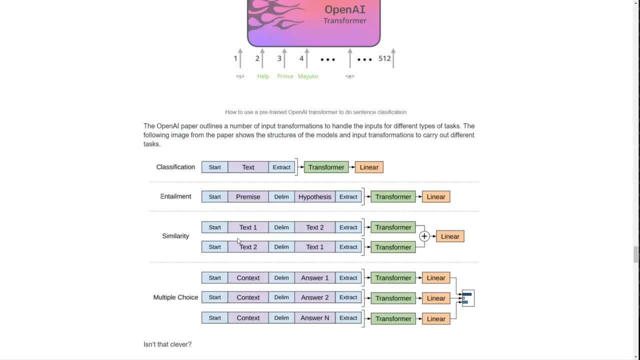 In the beginning you will use a spatial token called CLS And in the end you will use a spatial token called SAP, S-C-P or a separator. So he talks about all of that, I think, in this article. 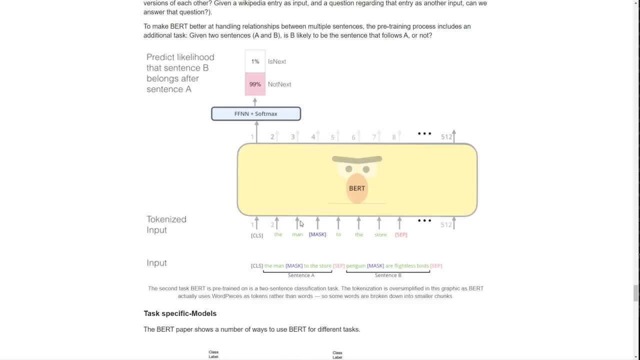 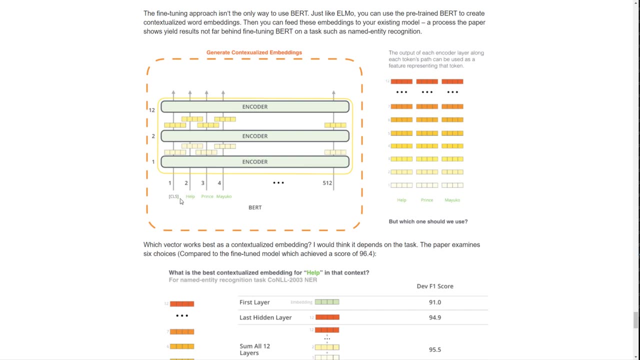 See CLS and mask. Actually CLS and We talked about the. I think we did not cover the mask language model, which we'll cover later. But see, like you have a word like this and it will generate the individual vector. 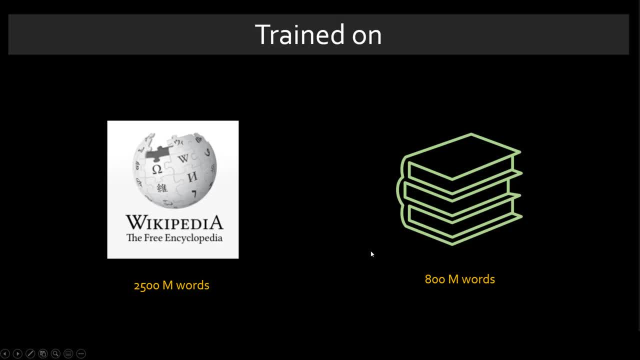 So you can go through this useful article. BERT was trained by Google on 2,500 million words in Wikipedia- 800 million words on different books. You know they look at different books and they generated this BERT. They trained the BERT using two approaches. 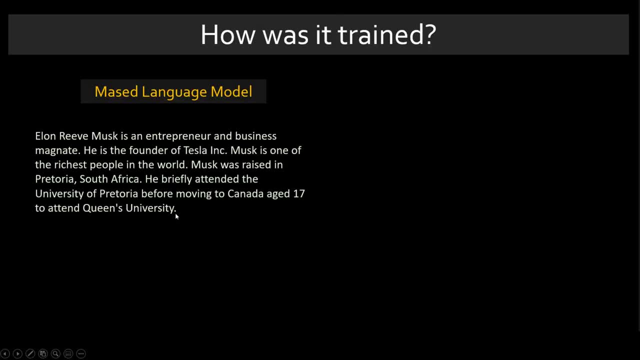 One is mask language model. So I have this Wikipedia article on Elon Musk, And what they did is they masked 15% of the words. For example, here there is entrepreneur, So they would just mask that And they would generate these training samples. 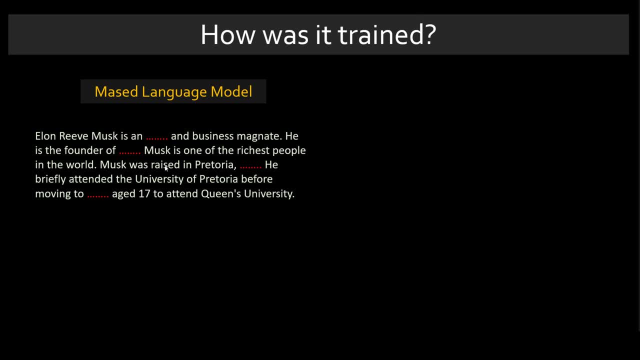 and they would train BERT model. Now, using this artificial task, when they train BERT model, as a side effect they are getting word embeddings. So really, the end purpose is to get word embeddings, But in order to get word embeddings, 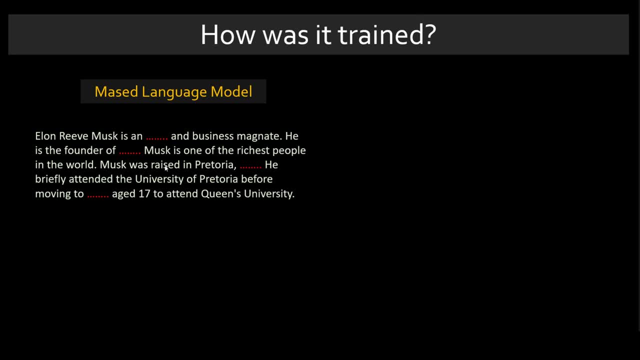 you have to train the- you know BERT model on artificial tasks. So the mask language model was really the artificial task that they used to train the model, But as a side effect you got meaningful word and sentence embedding. The other task that they trained on was: 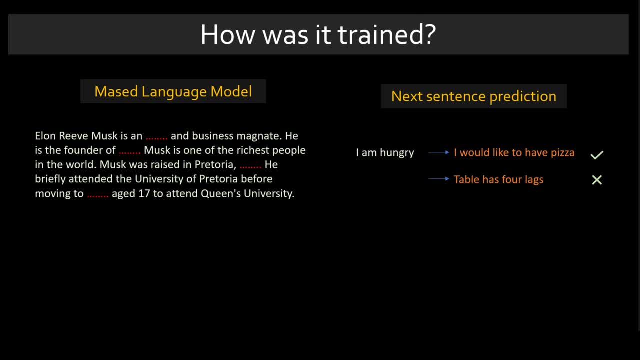 next sentence prediction. For example, if I say I am hungry, predict the next statement. If the next statement is: I would like to have pizza, The probability of that happening is more than you know. table has four legs. Who cares? I am hungry. 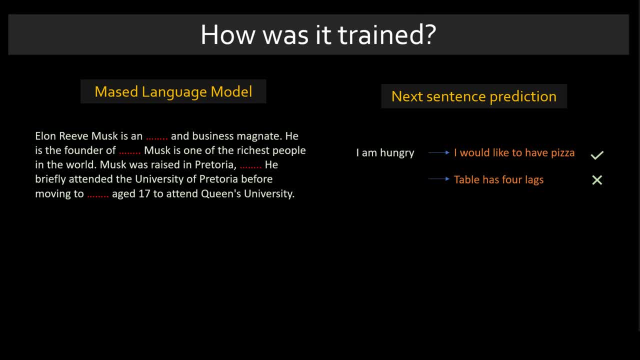 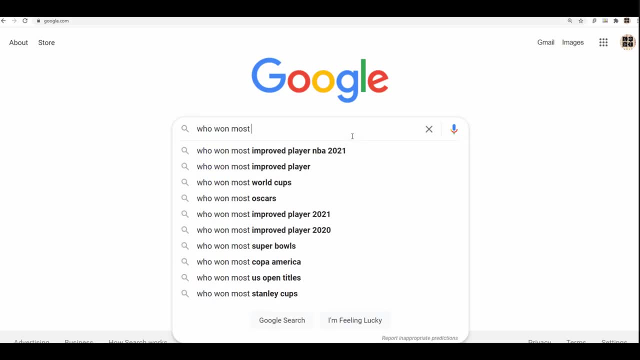 Give me some food Right, So the probability of that statement is very, very low. Using these two approaches, they train the BERT model, And today Google search is powered by BERT, So BERT has a direct impact on your life. 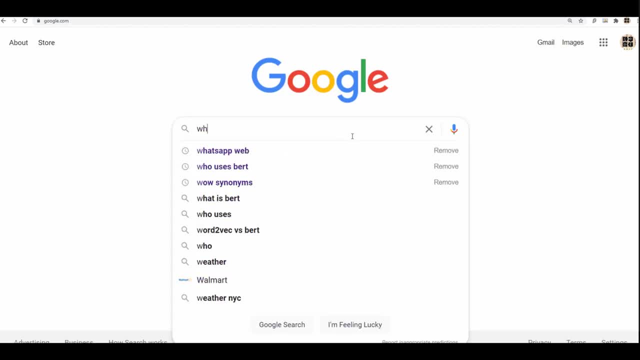 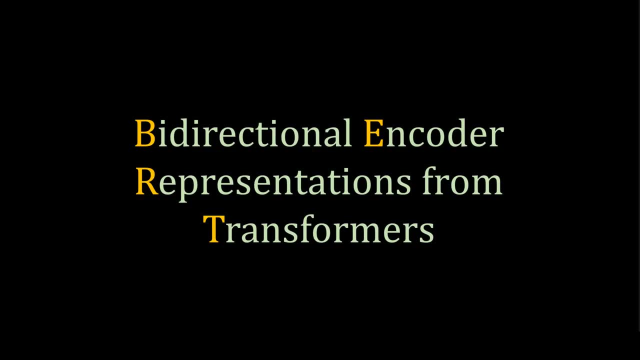 The search becomes more better in Google after they onboarded BERT in their search engine- The full form. here is the full form. if you're curious about what BERT means Now, let's look into TensorFlow code and we'll generate some sentence. 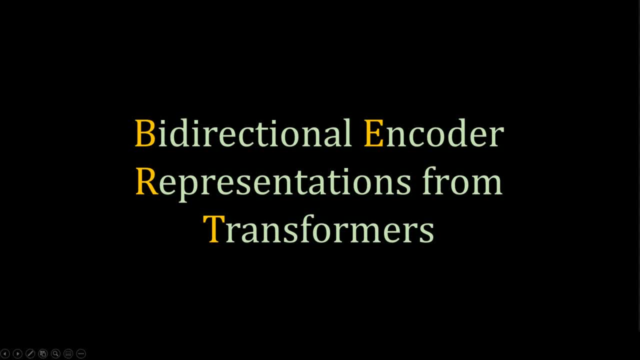 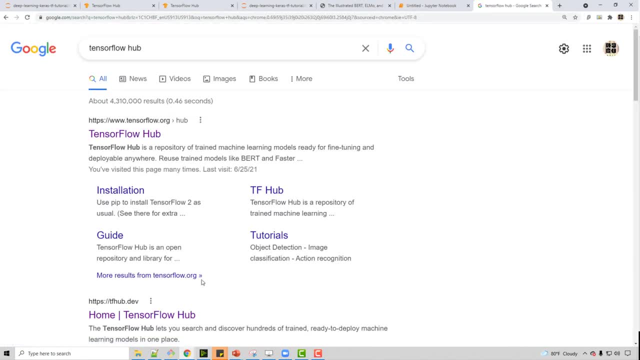 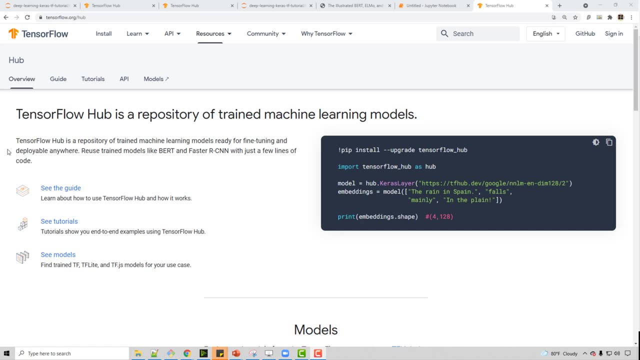 and some word embeddings in Python and TensorFlow. Let's try to locate the BERT model on TensorFlow Hub website. So if you Google TensorFlow Hub, you will go to the TensorFlow Hub, a repository of all the different models. And when you go see the models, 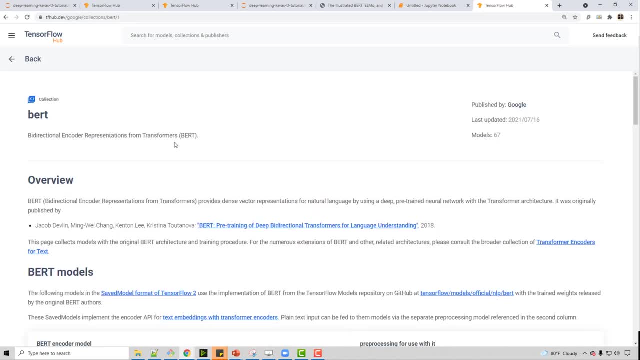 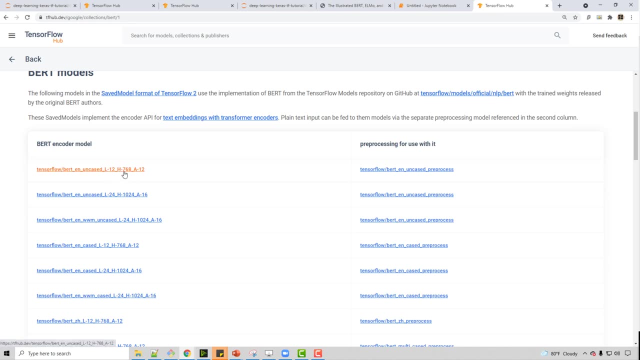 go here in embedding, you will see a section for BERT, And BERT has different models, you know, like L12.. This is like layer 12.. Hidden state 768.. Attention, 12.. This one is a bigger one. 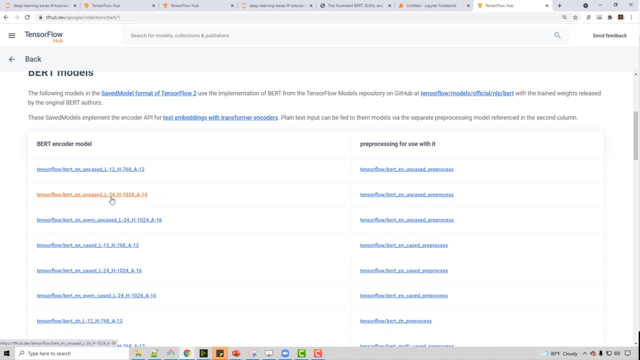 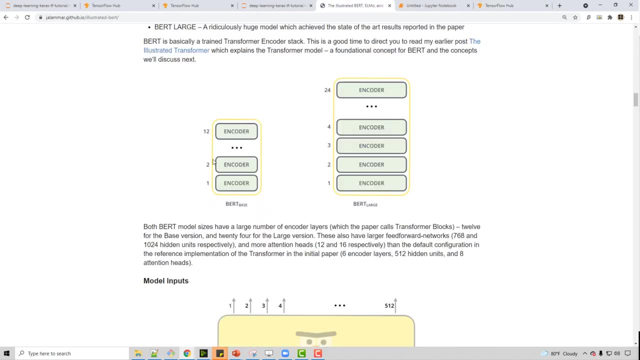 So there is a 12. So this is a BERT base And 24 is a BERT large. So if you read Jay Alamar's blog, it talks about BERT base, which has 12 encoders, and BERT large has 24.. 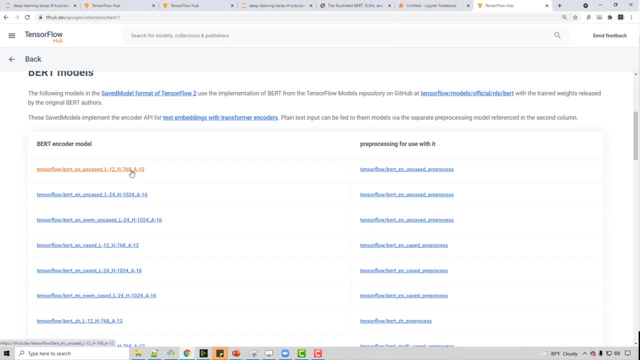 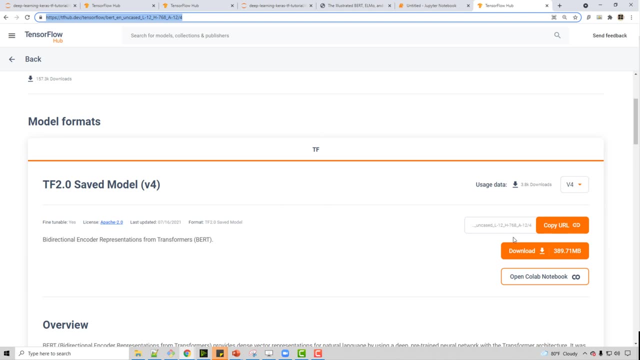 So we are going to use the basic encoder, basic BERT model, this one, And the good thing here is you can use this URL directly to download the model, or you can just copy it. See, it's 389 megabytes. 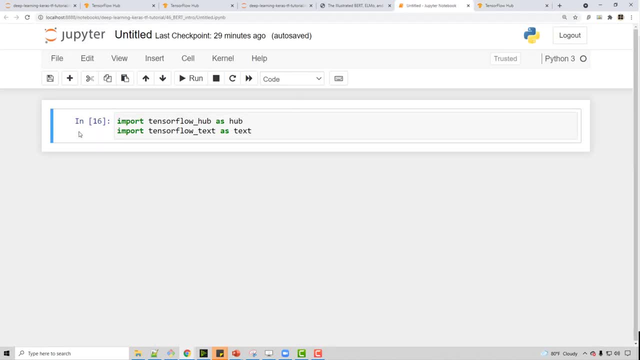 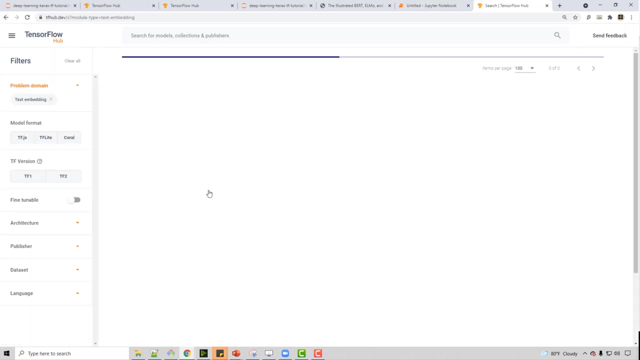 so it's going to take some time. So I'll just copy this URL here and I will create a variable called encoder URL And then for each of these models there is a corresponding preprocessing URL. So if you look at this table here, 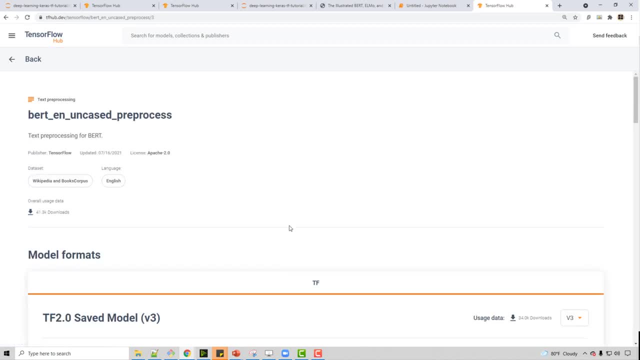 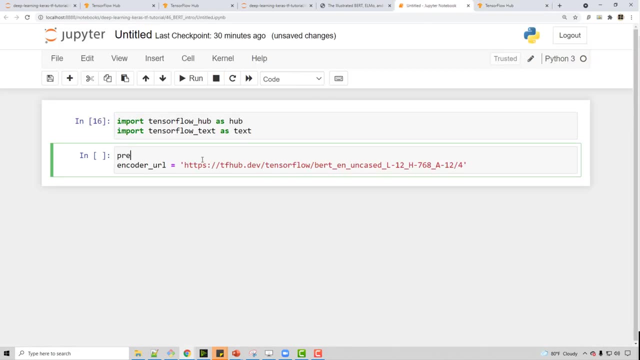 here there is a preprocessing URL. Now, preprocessing will preprocess your text. Okay, So I'm just going to copy it here. I'll just call it preprocess, Alright, So I have these two URLs. and now the next step for me. 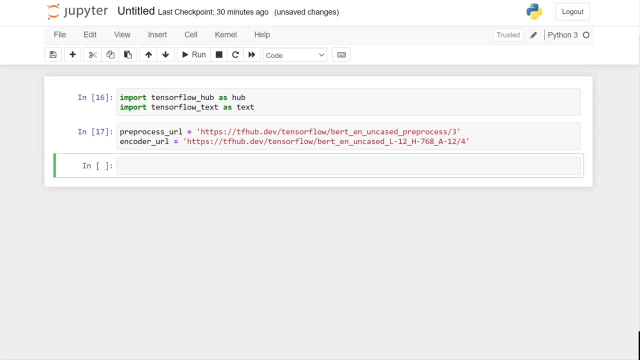 is to create hub. So hub is this hub. Okay, And you can out of this thing, you can create hub layer almost, And you can pass in your preprocess URL here And what it will give you is like a function pointer. 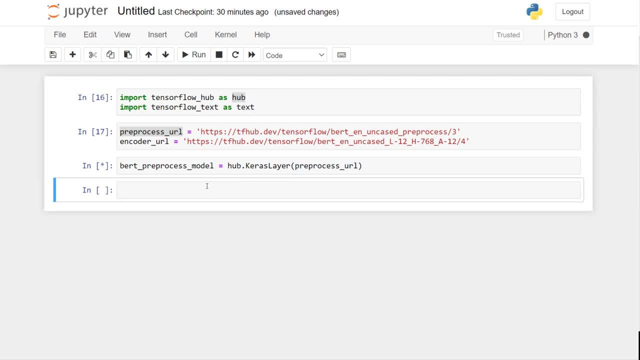 So I will call it BERT preprocess model And this you can treat it as a function pointer. You know, here you can supply some bunch of statements and it will do preprocessing on those statements. So let's say I'm building a 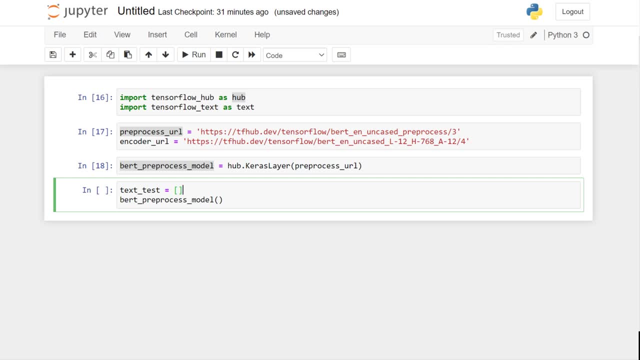 MUI classification model and I can have you know statement like this: Or I can have a different model and I might want to create word embedding or a sentence embedding for this statement. I love Python programming, Of course you do So now here. 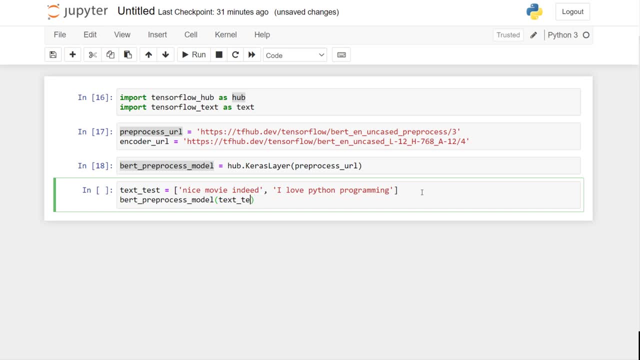 text test. So I will supply that into this and I will call the output object text preprocessed And it's going to be dictionary, Hence I will just print up you know keys, because the object might be big And it. 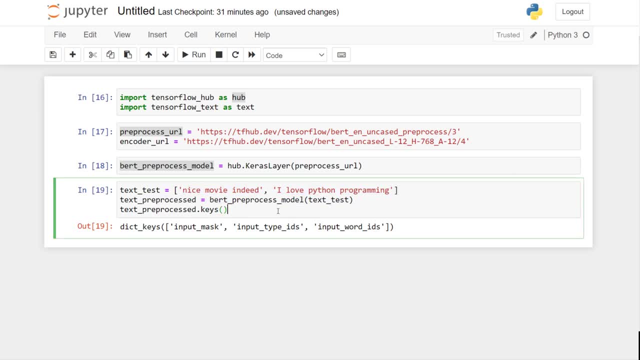 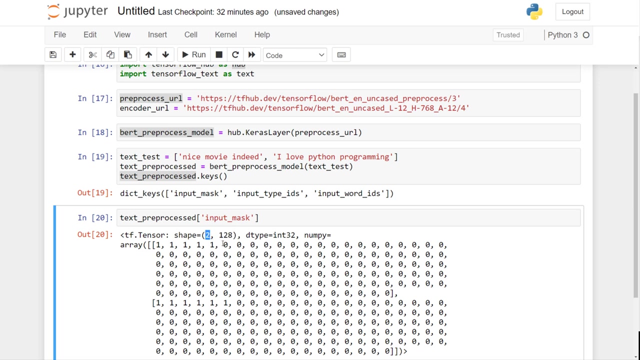 preprocessed these two sentences and it produced this particular object. So let's look at individual elements in this dictionary. The first one is input marks. Here the shape is 2 by 128.. 2 because we have two sentences. So for the 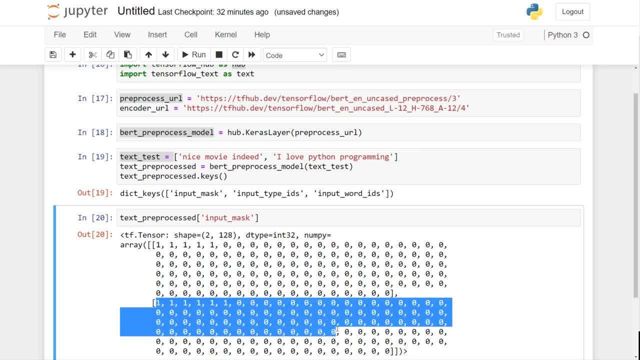 first sentence. this is the mask For the second one. this is the mask. Now, first sentence has three words, whereas the mask is five words. So what does it mean? All right, Let's try to understand that. So when 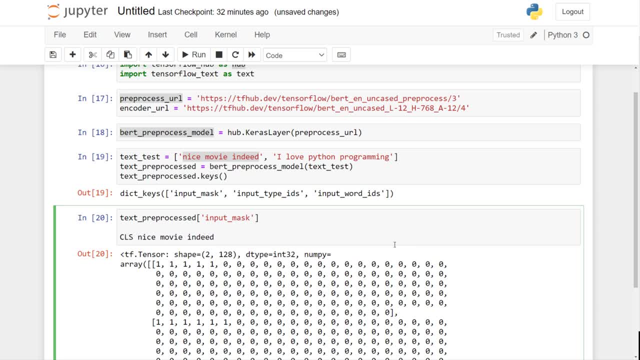 the way word works is, it will always put a special token called CLS in the beginning, And to separate two sentences it will put a special token called separator. So now, if you count tokens one, two, three, four, five, 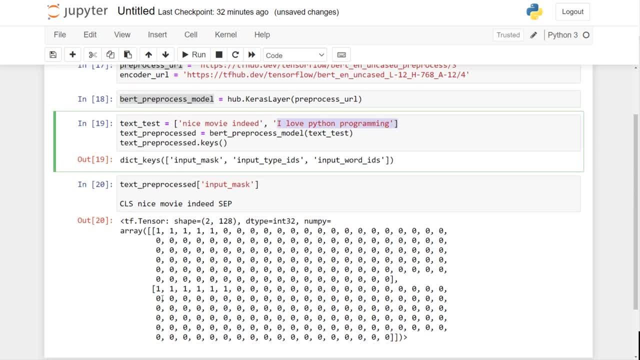 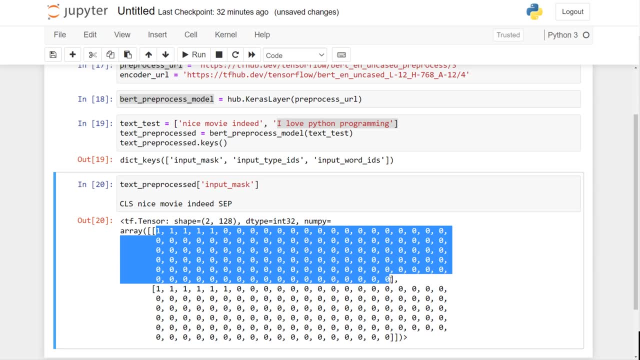 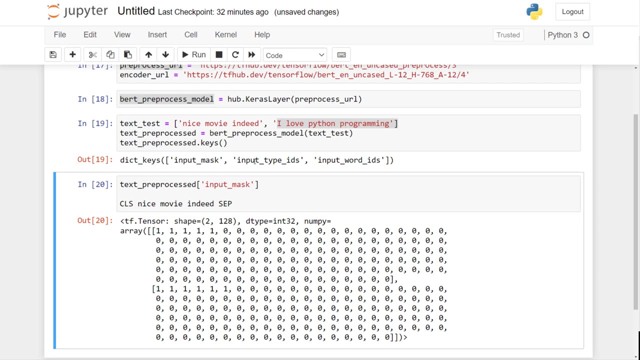 So see five And these are four, and four and two will be six, And 128 is a kind of like a maximum length of the sentence. So that's why you have 128 and remaining are zero, because you actually have only five words. 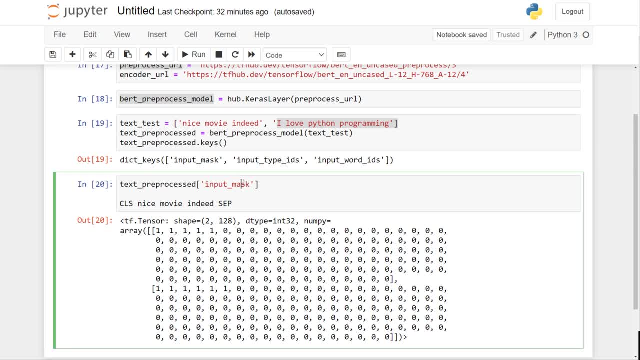 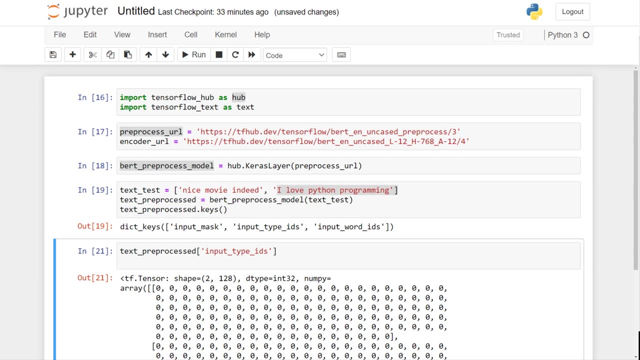 So input marks is pretty easy to understand. The input type IDs are really. they are really useful if you have multiple sentences in one statement. So you will see. for our use case everything is zero, So just don't worry too much. 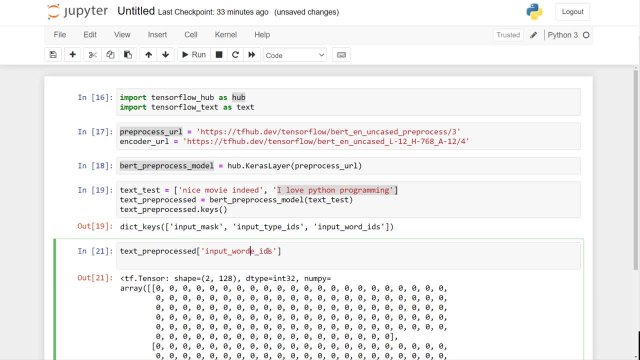 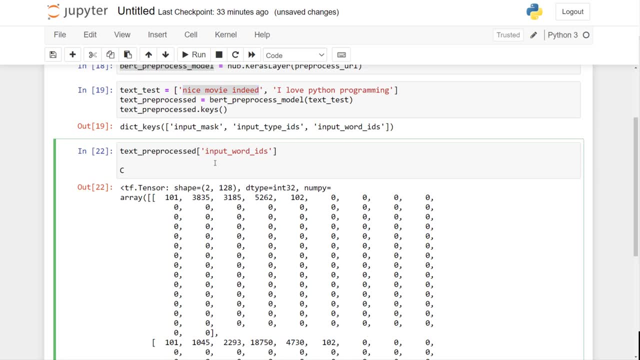 about it. Now let's look at input word IDs. All right, Again, I need to put this thing here. So there was special CLS statement in the beginning And in the end there was a separator statement and the word ID. 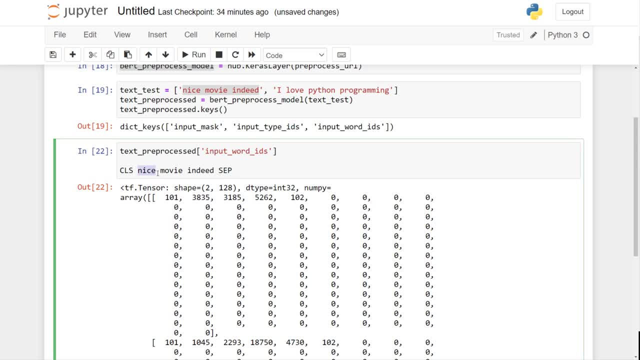 for separator is 102.. And these are the individual unique IDs for these words And these could be the IDs from a vocabulary. So this is part of the pre-processing stage. In the next stage we will actually create the word embeddings and 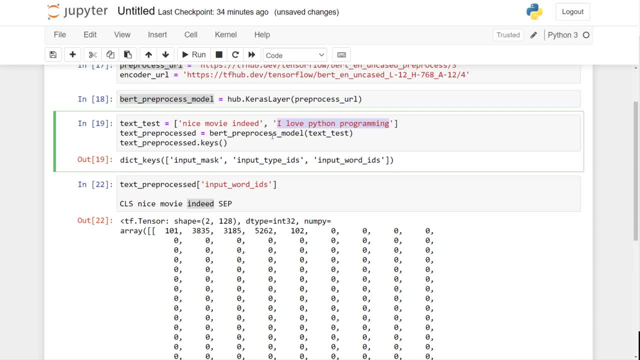 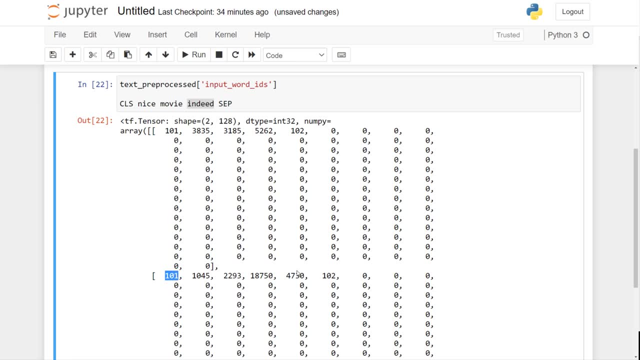 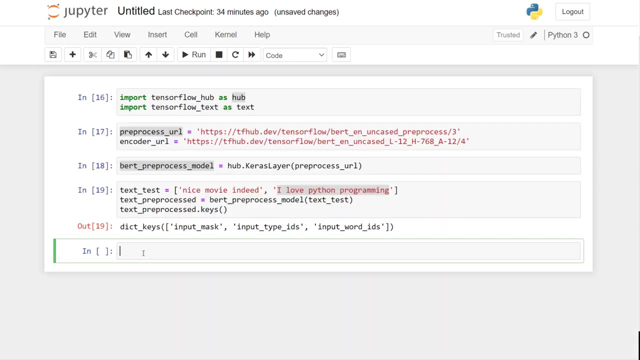 so on. This is for the first statement, which is nice movie indeed. The second statement is: I love Python programming, So this is the kind of the input word IDs for that. So this is the input word IDs for the first statement. 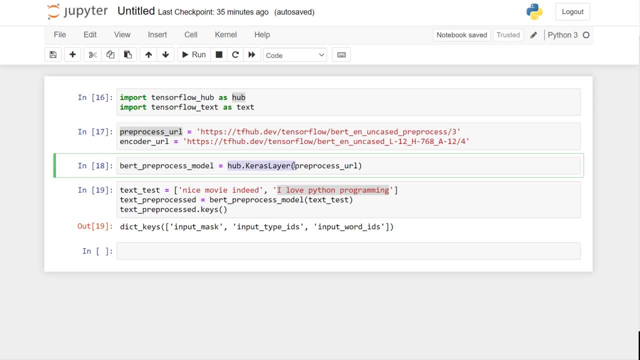 And then the third statement is to create another layer. So you will use the same function here. You will create another layer, So I will just copy paste this one, And the another layer will have encoder URL. okay, So the 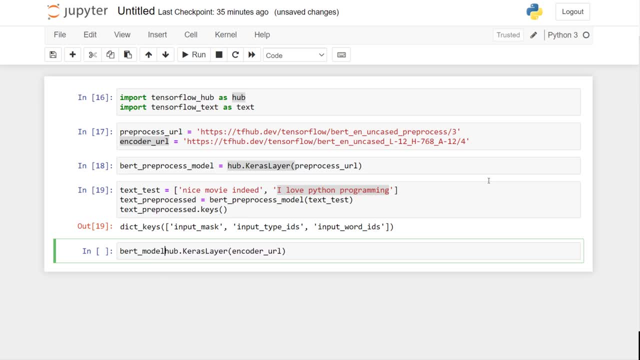 encoder will call it bird model. let's say Okay, And the bird model will act like a function pointer, just like what we did before. So now you can treat it as a function pointer, almost like a function, And you can. 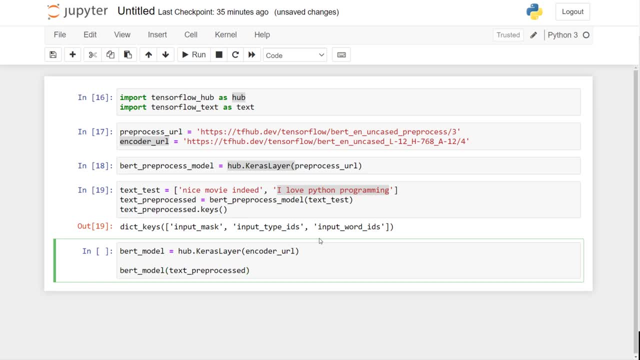 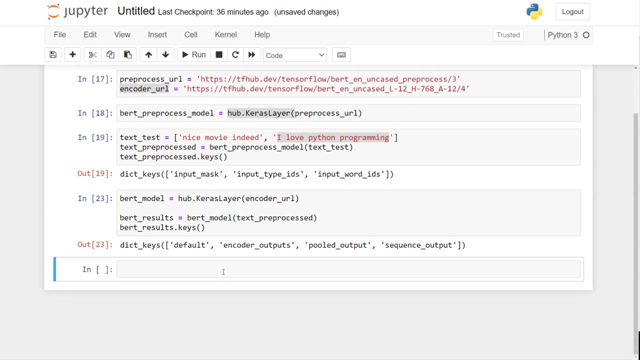 supply your preprocess text So you can use the word embedding to store that into this particular object And I will call this is a dictionary. so I will try to get the keys of that dictionary. It's going to take some time but 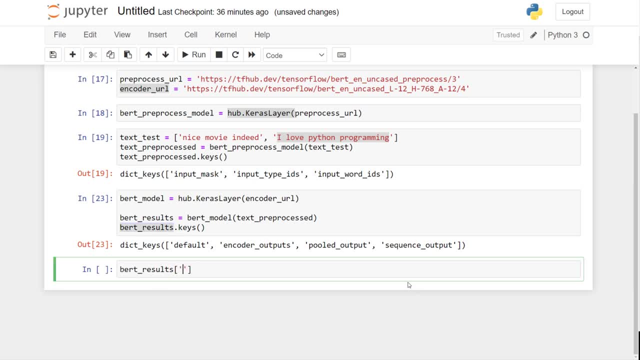 it will come back at some point, All right. So this is an embedding for the entire sentence. We have two sentences. So for nice movie, indeed, this is the embedding, And the embedding vector size is 768.. So this, 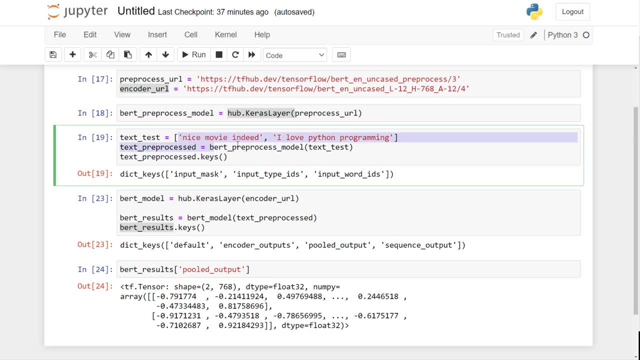 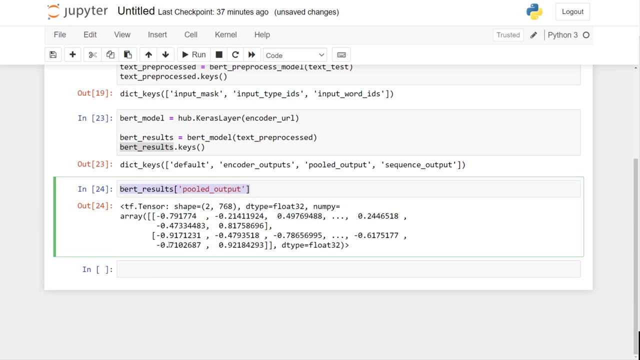 768 vector accurately represents the statement nice movie, indeed, in form of numbers. Similarly, for the second sentence, you can use these vectors in your natural language processing task. It could be movie review, classification, name, entity recognition. it could be anything But. 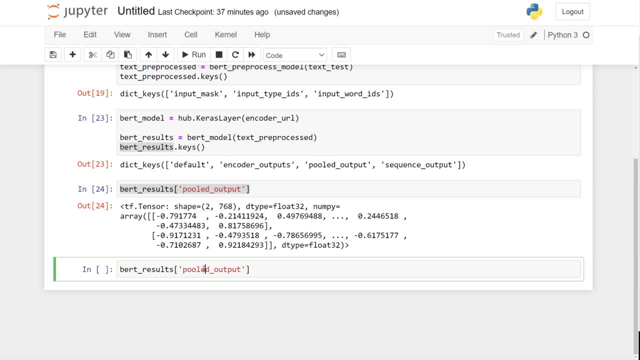 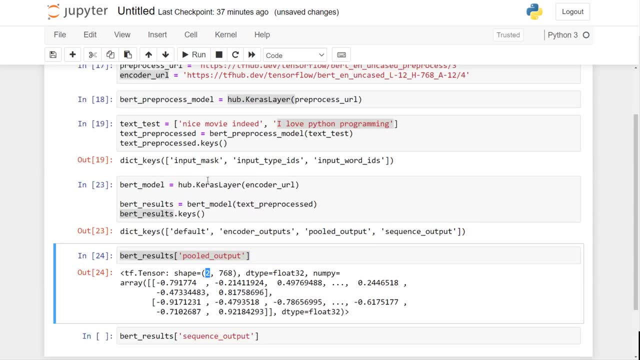 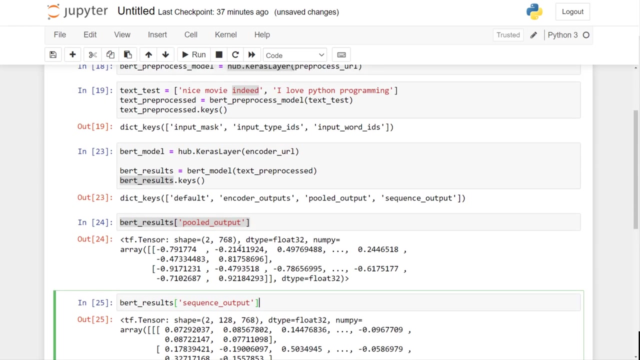 BERT helps you generate a meaningful vector out of your statement. Now, for each sentence, for each of these words, it will have 768 size vector. So see, size is 2 by 128.. Why 128? Because 2 is. 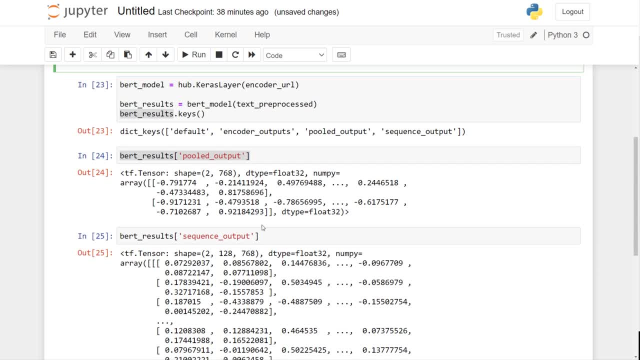 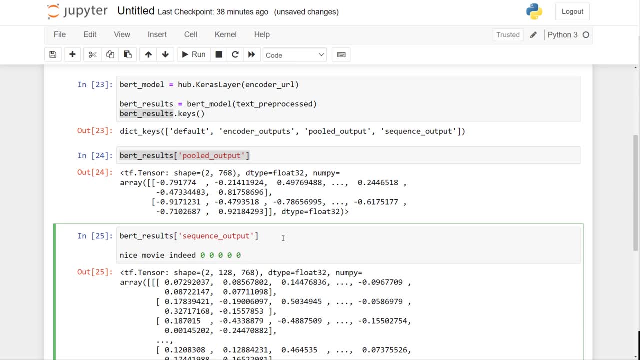 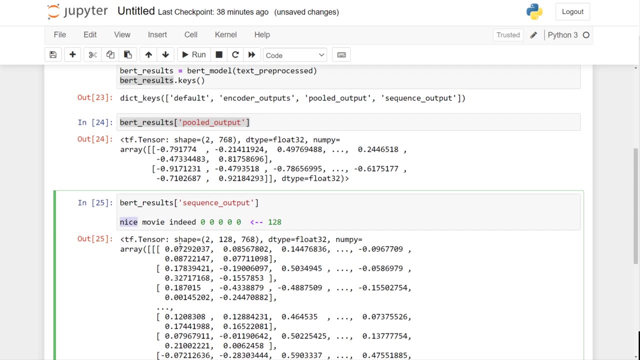 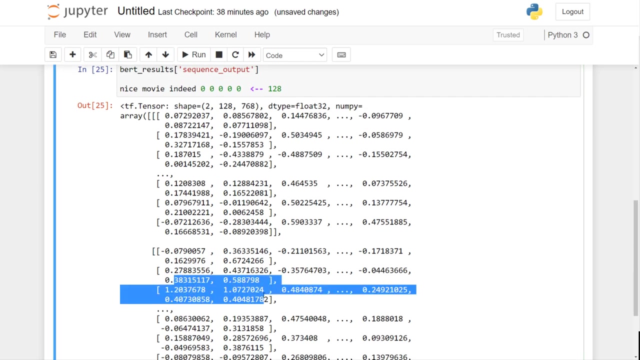 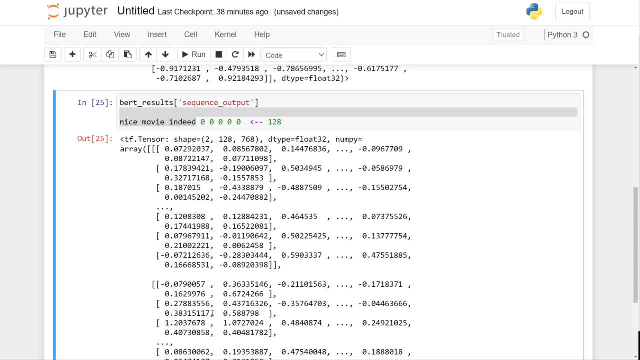 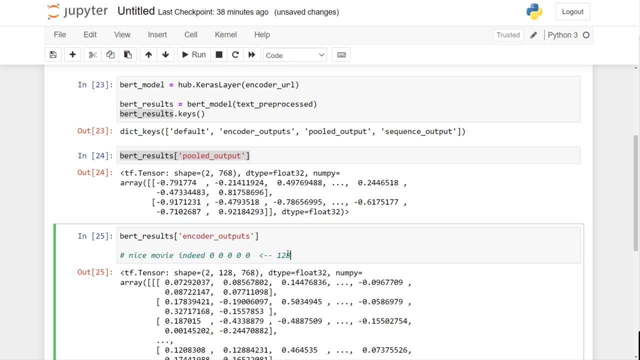 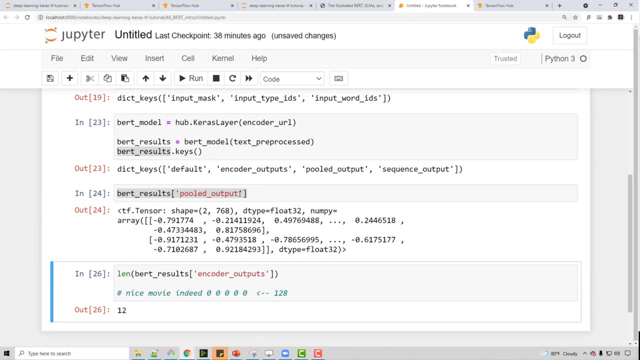 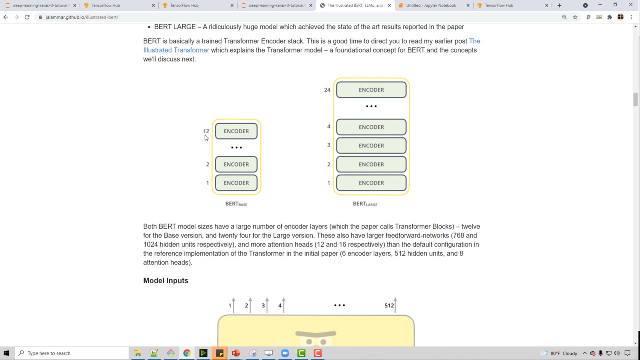 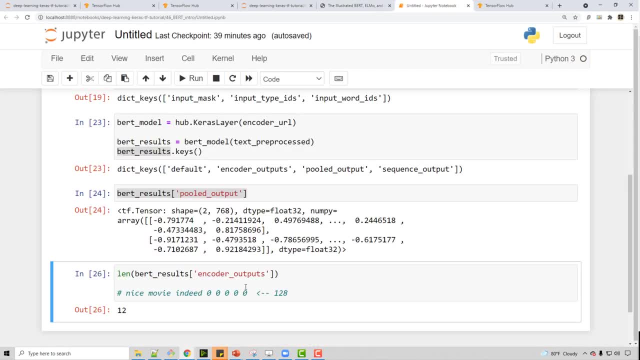 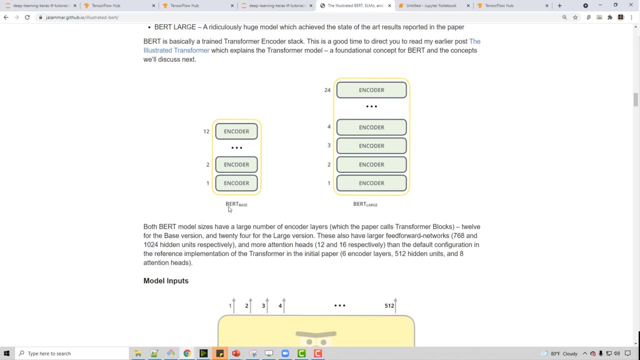 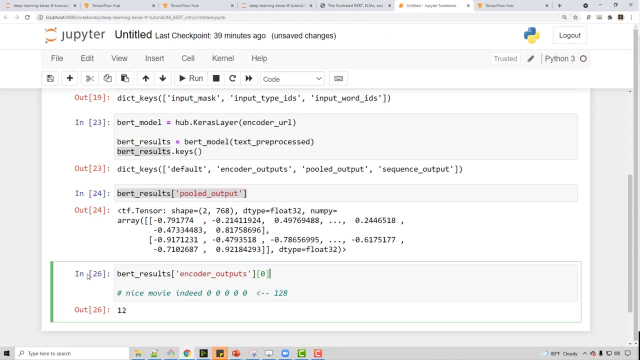 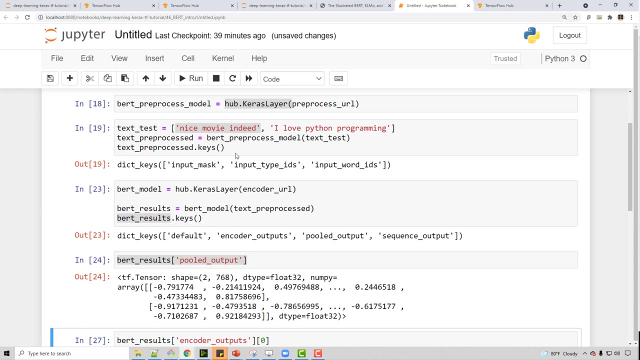 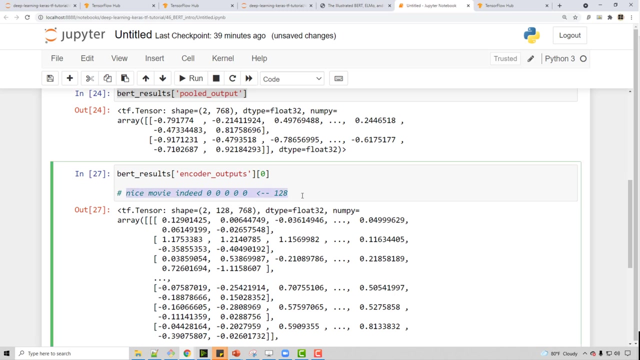 this is 12 is because we have two sentences, So these encoder outputs is nothing but the output of each individual encoder, So we have 12.. That's why 12 is the size And each of them. let's see if.